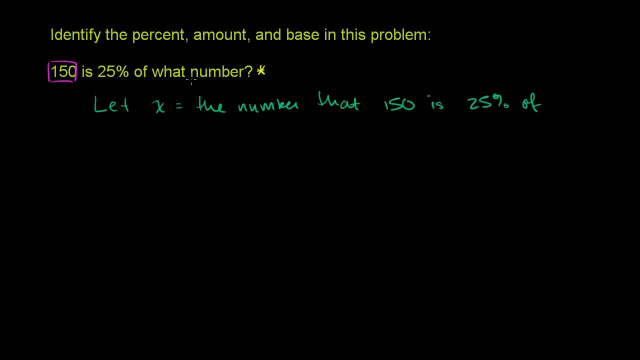 That's what we need to figure out. 150 is what is 25% of what number? That number right here we're seeing is x. So that tells us that if we start with x and if we were to take 25% of x, you could imagine that's the same thing. 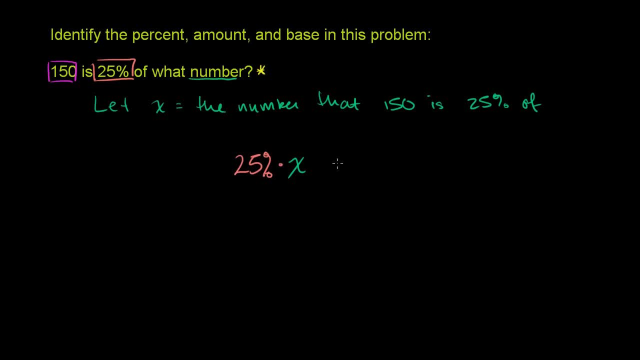 as multiplying it by 25%, which is the same thing as multiplying it if you view it as a decimal, times 0.25, times x. These two statements are identical. So if you start with that number, you take 25% of it, or? 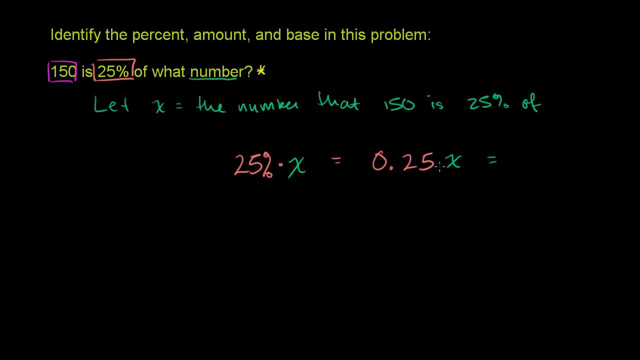 you multiply it by 0.25, that is going to be equal to 150.. 150 is 25% of this number, And then you can solve for x. So let's just start with this one over here. So if we just have, let me just write it separately. so 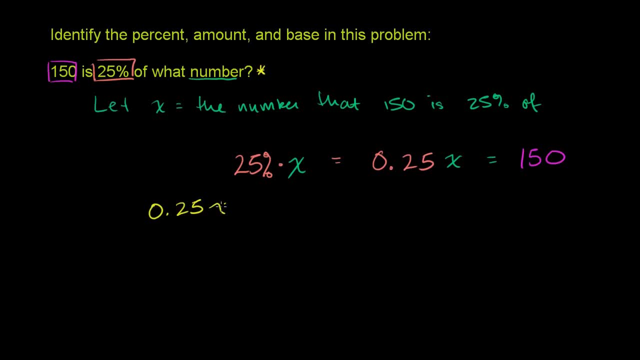 you understand what I'm doing. 0.25 times some number is equal to 1.25.. 150.. Now there's two ways we can do this. We can divide both sides of this equation by 0.25, or if: 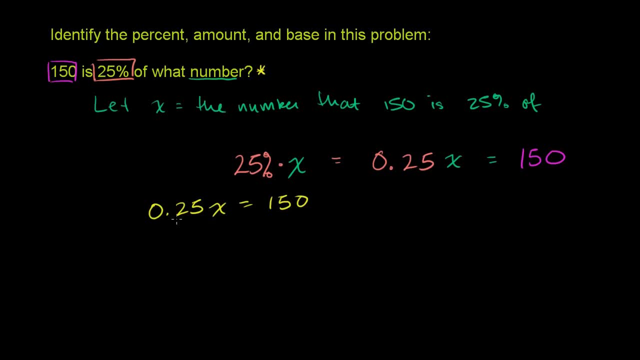 you recognize that well, you know, 4 quarters make $1, you could say: let's multiply both sides of this equation by 4.. You could do either one. I'll do the first, because that's how we normally do. 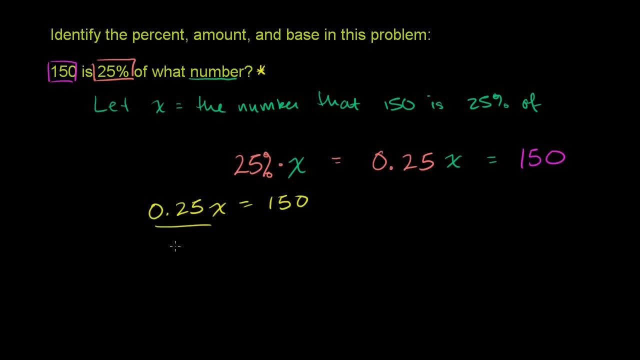 algebra problems like this. So let's just multiply both by 0.25, multiply this times or multiply it by 0.25.. 0.25., 0.25. 0.25. 0.25. 0.25.. 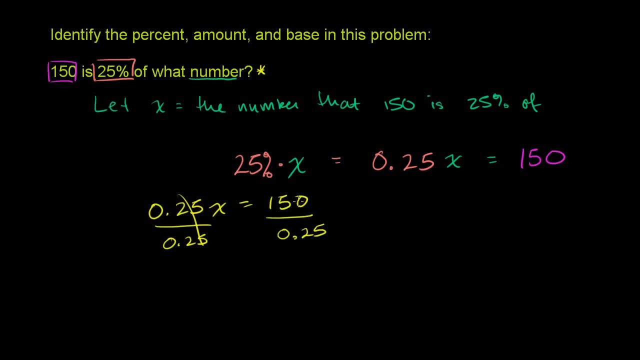 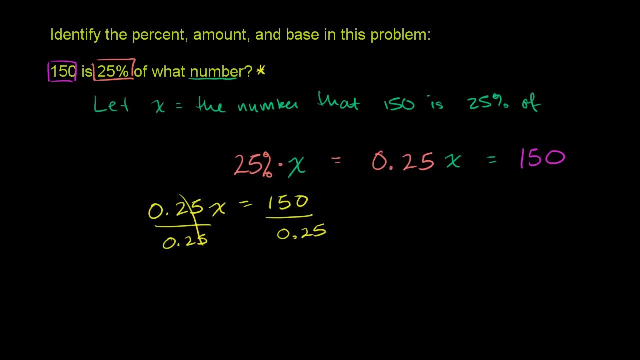 And the reason why I wanted to do this is really: is this good practice, dividing by a decimal? So let's do that. So we want to figure out what 150 divided by 0.25 is, And we've done this before. 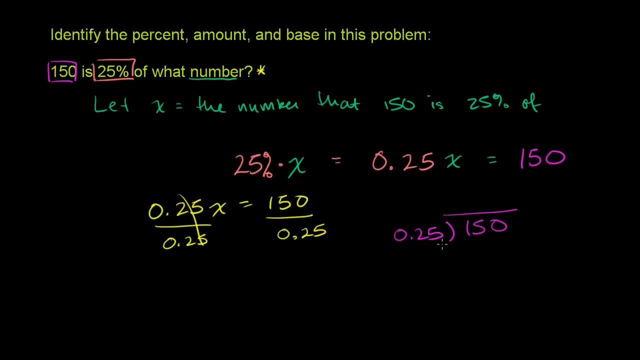 When you divide by a decimal, what you could do is you can make the number that you're dividing into the other number. you could turn this into a whole number by essentially shifting the decimal 2 to the right. But if you do that for the number in the denominator you 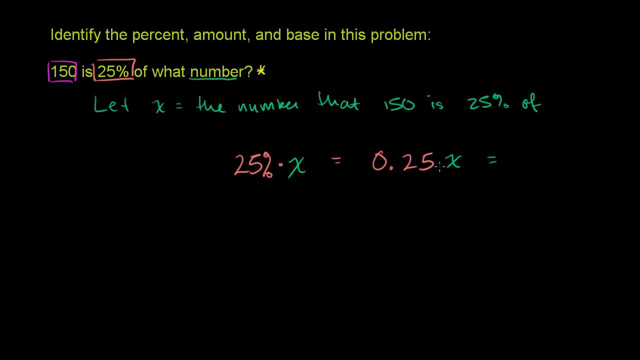 you multiply it by 0.25, that is going to be equal to 150.. 150 is 25% of this number, And then you can solve for x. So let's just start with this one over here. So if we just have, let me just write it separately. so 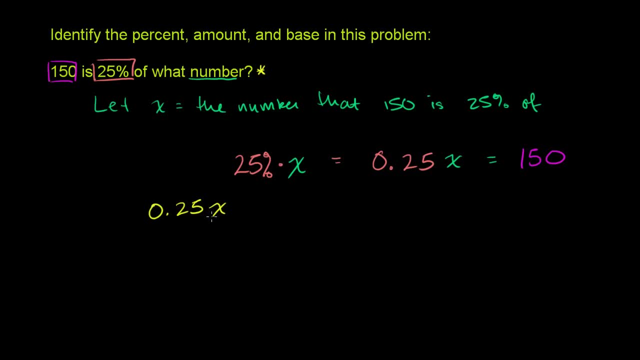 you understand what I'm doing. 0.25 times some number is equal to 1.25.. 150.. Now there's two ways we can do this. We can divide both sides of this equation by 0.25.. Or, if you recognize that well, you know 4 quarters. 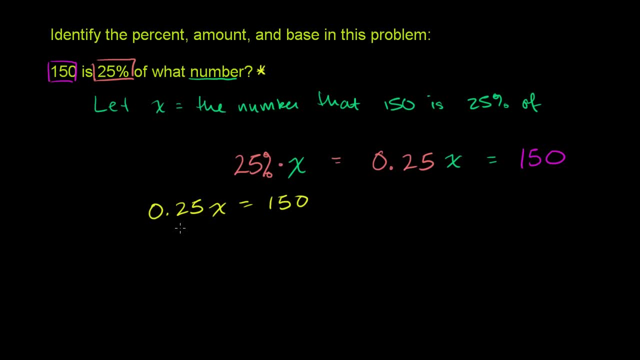 make $1,. you could say: let's multiply both sides of this equation by 4.. You could do either one. I'll do the first, because that's how we normally do algebra problems like this. So let's just multiply both by 0.25.. 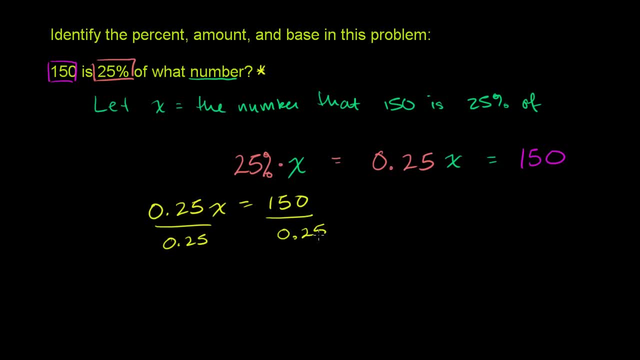 Multiply this times, or multiply it by 0.25, that will just be an x, And then the right-hand side will be 150 divided by 0.25.. And the reason why I want to do this is really: is this good? 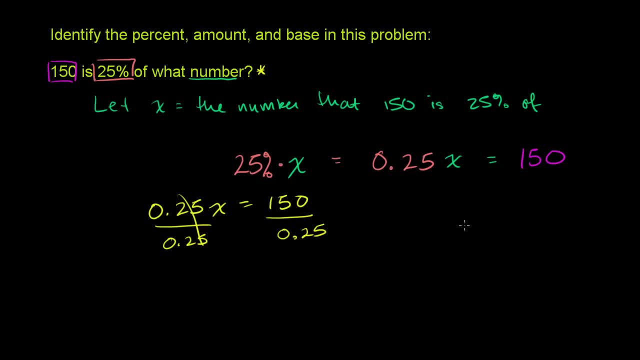 practice dividing by a decimal. So let's do that. So we want to figure out what 150 divided by 0.25 is, And we've done this before. When you divide by a decimal, what you can do is you can make the number that you're dividing into the other number. 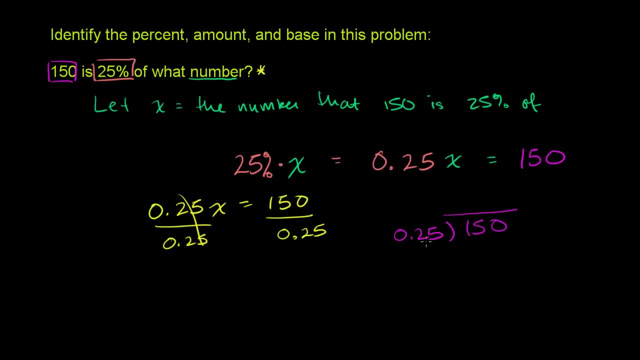 you can turn this into a whole number by essentially shifting the decimal 2 to the right. But if you do that for the number in the denominator it's going to be 0.25.. You also have to do that to the numerator. 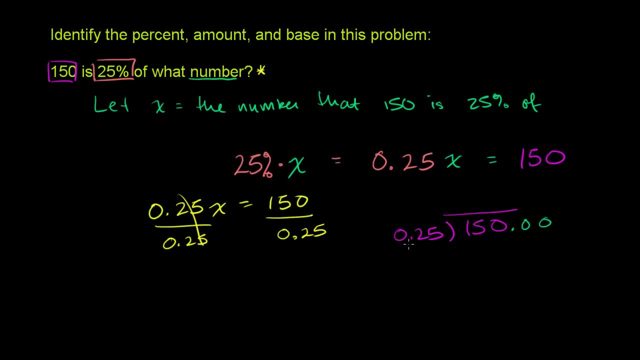 So right now you could do this as 150.00.. If you multiply 0.25 times 100, you're shifting the decimal 2 to the right. Then you'd also have to do that with 150.. So then it becomes 15,000. 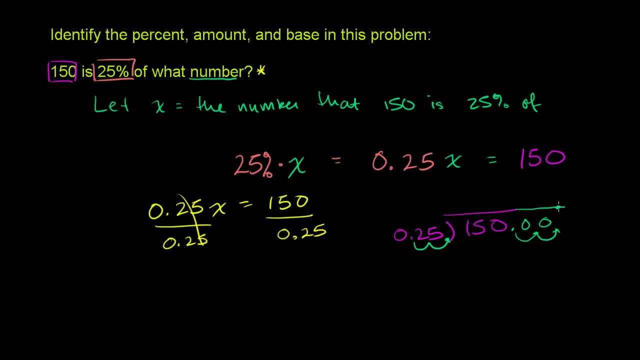 Shift it 2 to the right, So our decimal place becomes like this: So 150 divided by 0.25 is the same thing as 15,000 divided by 25.. And let's just work it out really fast. So 25 doesn't go into 15,000. 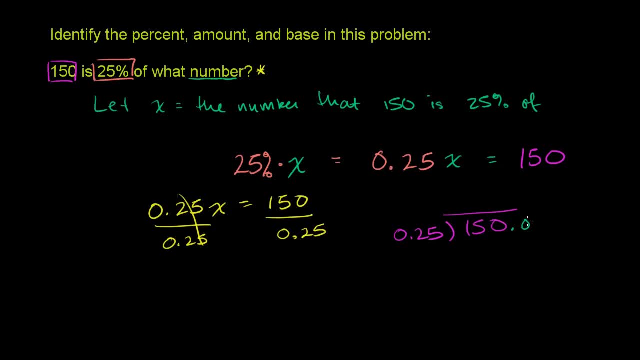 We'd also have to do that to the numerator. So right now you could do this as 150.00.. If you multiply 0.25 times 100, you're shifting the decimal 2 to the right. Then you'd also have to do that with 150. 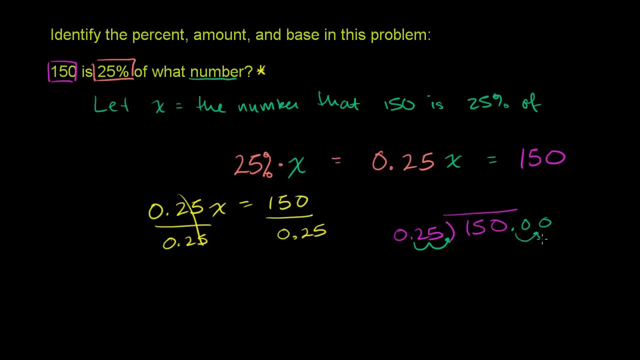 So then it becomes 15,000.. Shift it 2 to the right, So our decimal place becomes like this: So 150 divided by 0.25 is the same thing as 15,000 divided by 25.. And let's just work it out really fast. 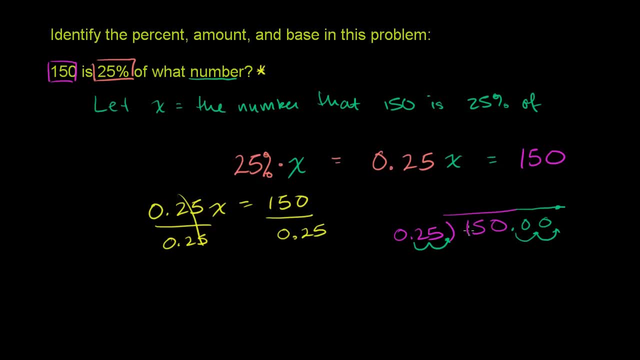 So 25 doesn't go into 1,, doesn't go into 15.. It goes into 150, what is that 6 times right? It goes into 104 times. It goes into 150. 6 times 6 times 0.25 is, or actually this is now a 25.. 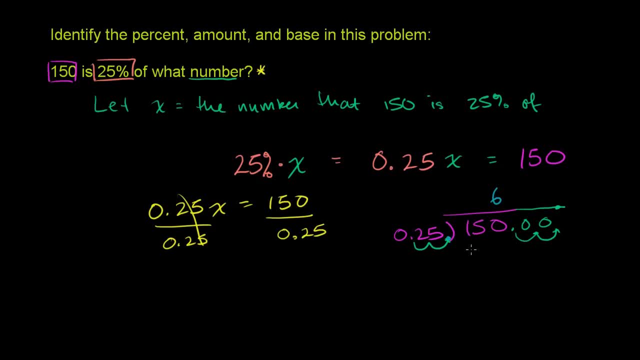 We've shifted the decimal, The decimal's sitting, right over there. So 6 times 25 is 150.. You subtract, You get no remainder. Bring down this 0 right here. 25 goes into 0.. 0.. 0. 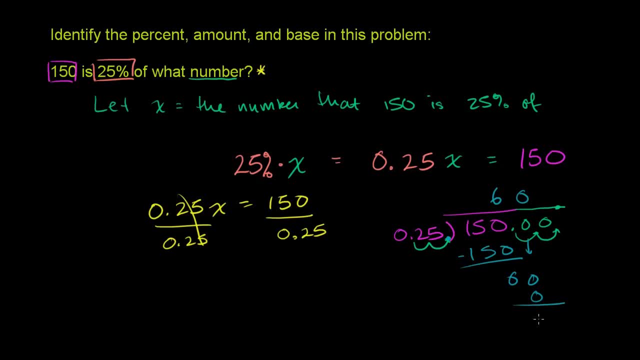 0.. 0 times 0 times 25 is 0.. Subtract- No remainder. Bring down this last: 0.. 25 goes into 0.. 0 times 0 times 25 is 0.. Subtract- No remainder. 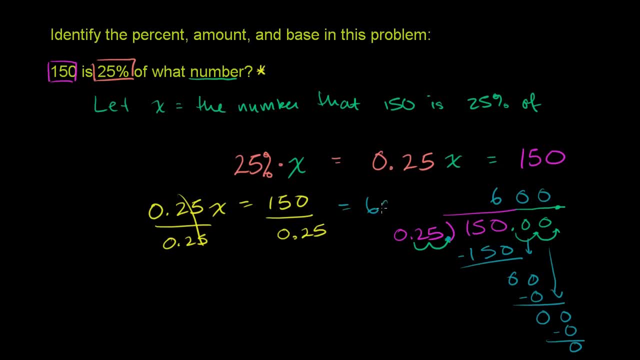 So 150 divided by 0.25 is equal to 600.. And you might have been able to do that in your head, Because when we were at this point in our equation, 0.25x is equal to 150, you could have just multiplied both sides. 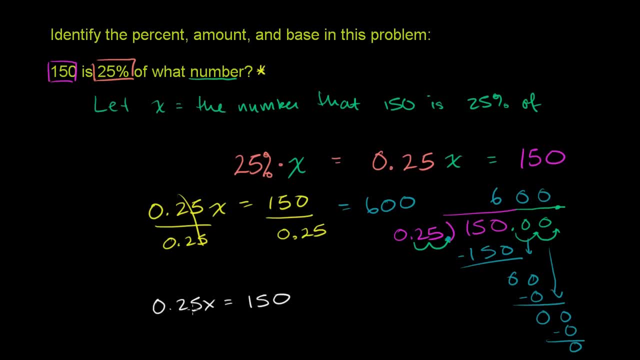 of this equation times 4.. 0.25 is the same thing as 4 times 1, 4th, which is a whole, And 4 times 150 is 600.. So you would have gotten it either way And this makes total sense. 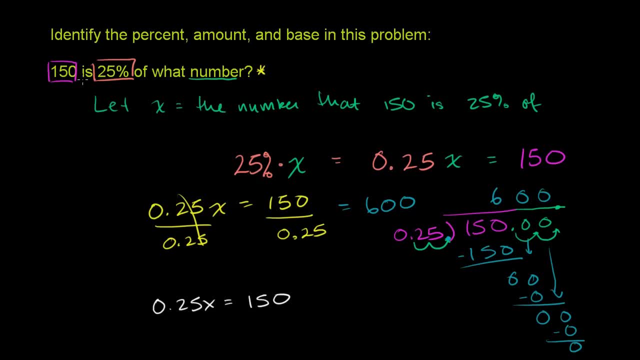 Because if 150 is 25% of some number, that means 150 should be 1 4th of that number. It should be a lot smaller than the number And it is. 150 is 1 4th of 600.. 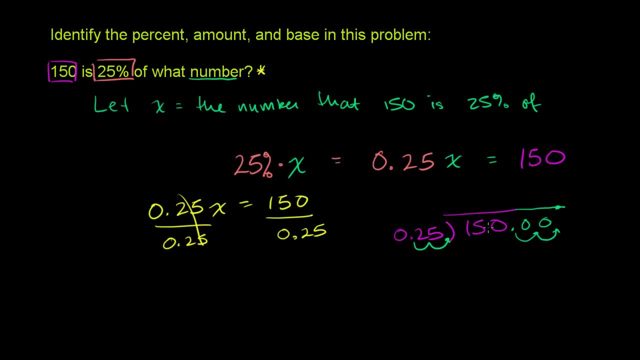 It doesn't go into 1.. It doesn't go into 15.. It goes into 150, what is that? 6 times right? It goes into 104 times. It goes into 150. 6 times 6 times 0.25 is, or actually this is now a 25.. 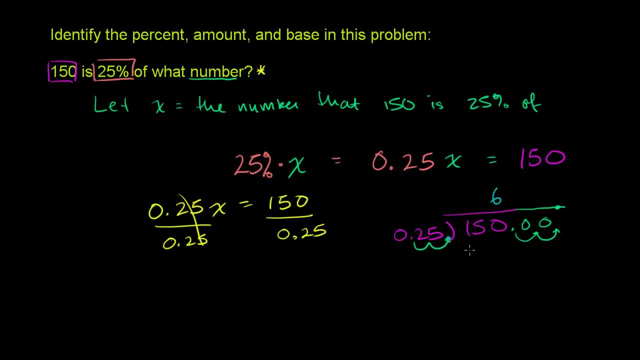 We've shifted the decimal, The decimal's sitting, right over there. So 6 times 25 is 150.. You subtract, You get no remainder. Bring down this 0 right here. 25 goes into 0, 0 times 0 times 25.. 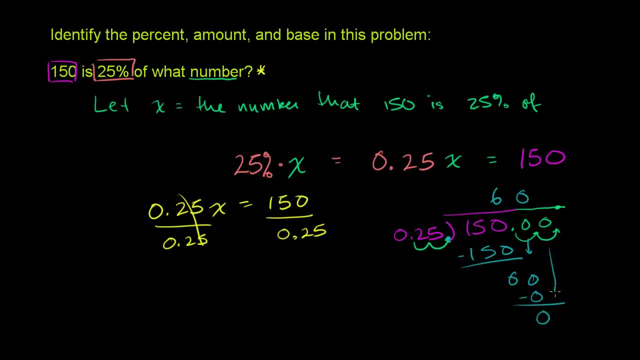 25 is 0.. Subtract: No remainder. Bring down this last 0.. 25 goes into 0. 0 times 0 times 25 is 0.. Subtract: No remainder. So 150 divided by 0.25 is equal to 600. 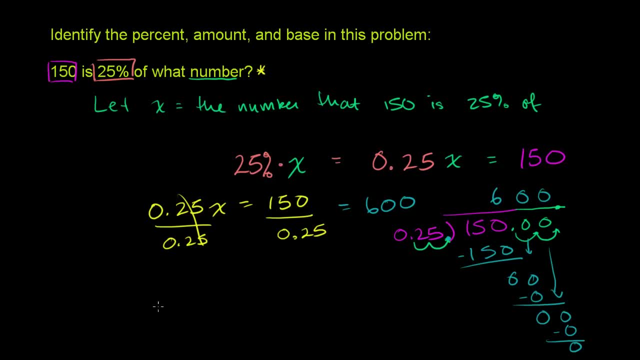 And you might have been able to do that in your head, Because when we were at this point in our equation, 0.25x is equal to 150.. You could have just multiplied both sides of this equation times 4.. 4 times 0.25 is the same thing as 4.25.. 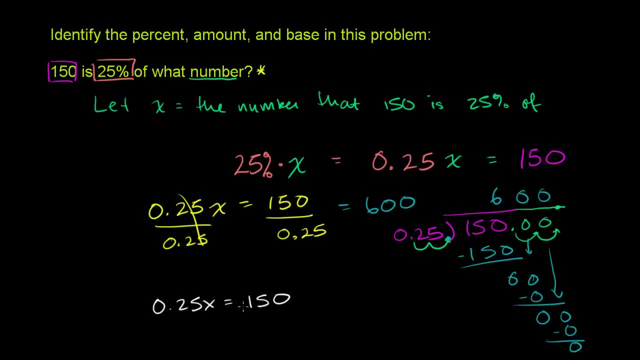 It's the same thing as 4 times 1, 4th, which is a whole, And 4 times 150 is 600.. So you would have gotten it either way, And this makes total sense, Because if 150 is 25% of some number, that means 150 should. 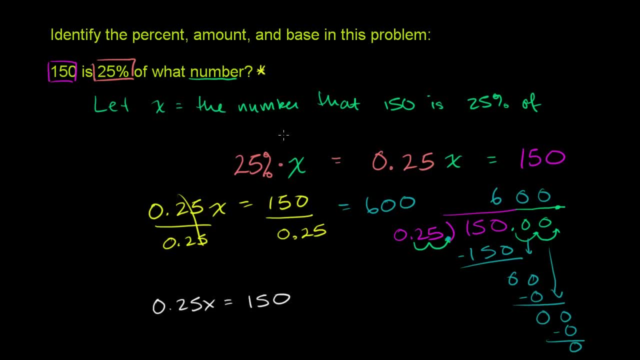 be 1 4th of that number. It should be a lot smaller than the number And it is. 150 is 1 4th of 600.. Now let's answer their actual question. Identify the percent. Well, it looks like 25%. 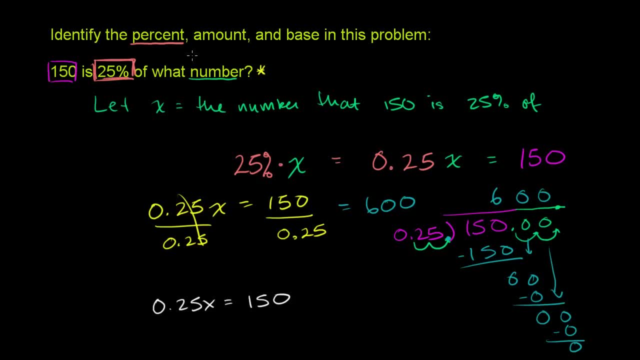 Identify the percent. Well, it looks like 25%. That's the percent. is 25% The amount and the base? in this problem, And based on how they're wording it, I assume amount means when you take the 25% of the base. so they're saying: 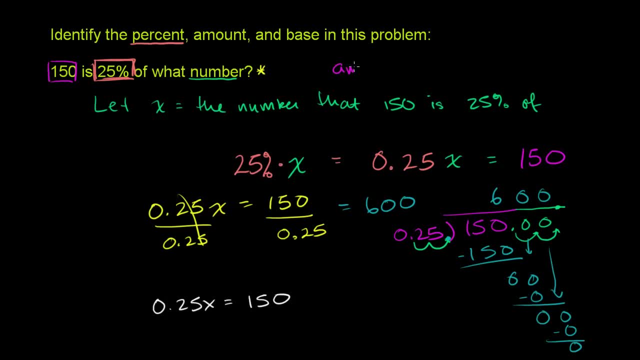 that the amount is. my best sense of it is that the amount is equal to the percent times the base. Let me do the base in green. So the base is 25%. The base is the number you're taking the percent of. 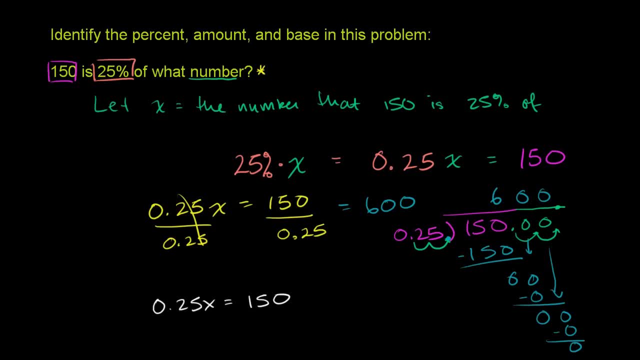 Now let's answer their actual question: Identify the percent. It looks like 25%, That's the percent. is 25% The amount and the base in this problem And based on how they're wording it, I assume amount means when you take the 25% of the base.